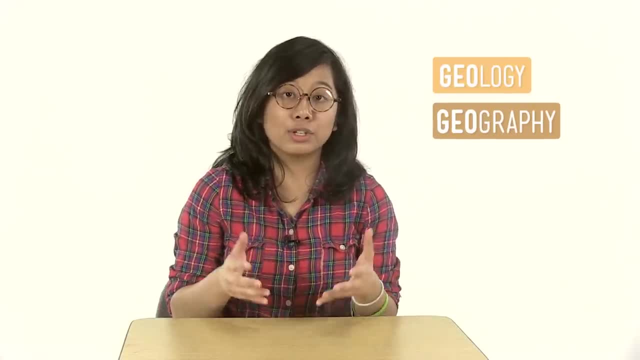 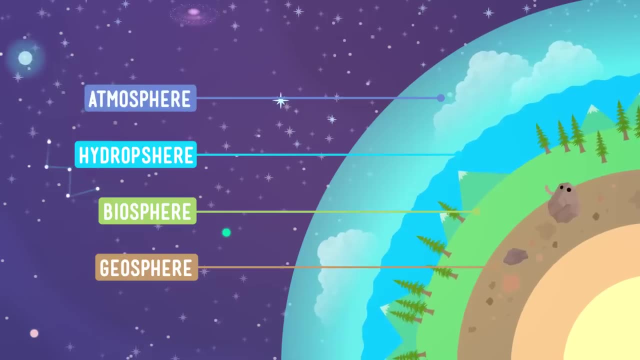 geology or geography. It basically means having to do with the Earth And in a way, the geosphere is kind of like the skeleton of our planet. All of the other spheres are built on top of it. It's made up of all the rocks and minerals on Earth, from the biggest boulders to the 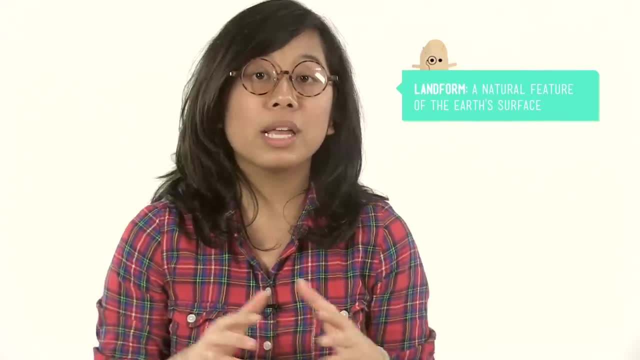 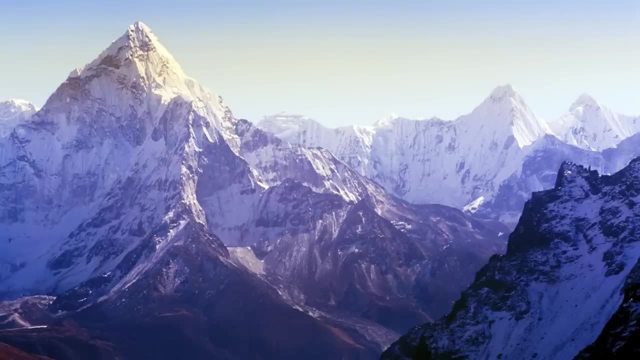 tiniest grains of sand And all of the landforms that those rocks and minerals make up are part of the geosphere too. I'm talking volcanoes, canyons, beaches, mountains and mountains, You name it. If it's made out of solid Earth, it's part of the geosphere. 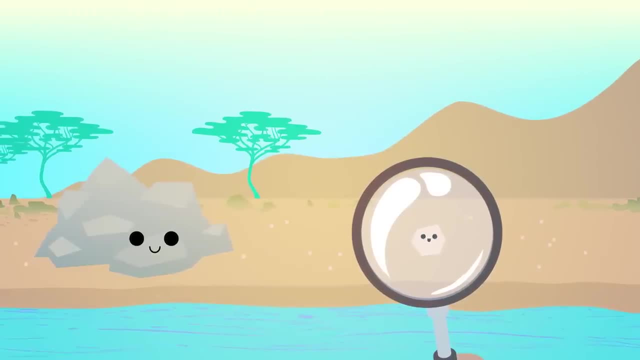 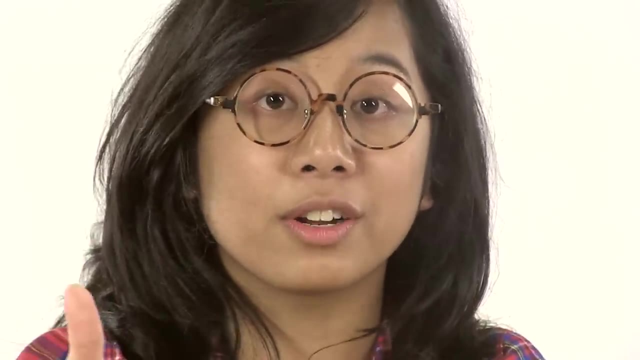 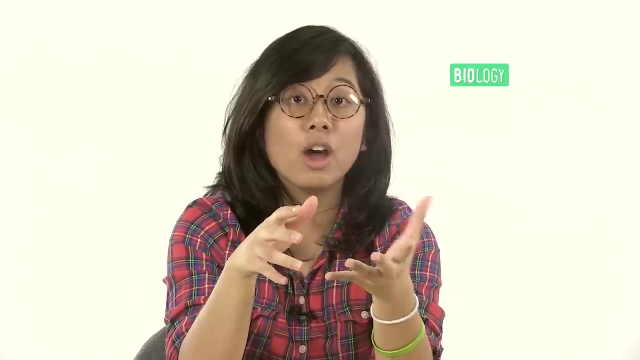 Now it's important to remember that the geosphere includes only non-living stuff. Living things do need to eat, though, And all living things are part of another one of Earth's spheres, the biosphere. Bio is Greek for life, And like geo, you've probably heard it before in words like biology. 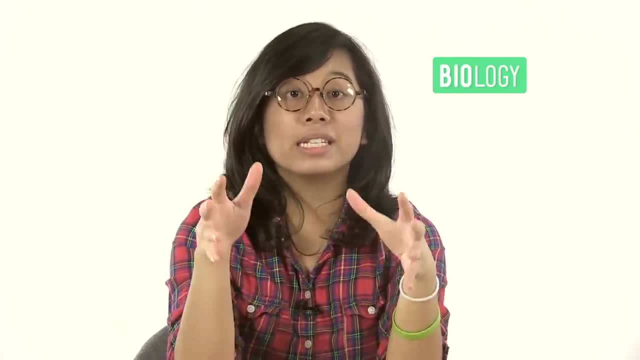 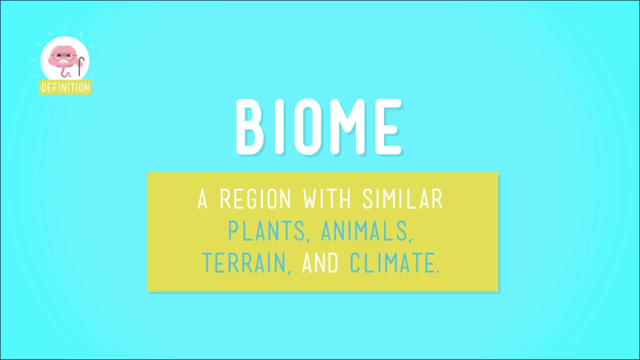 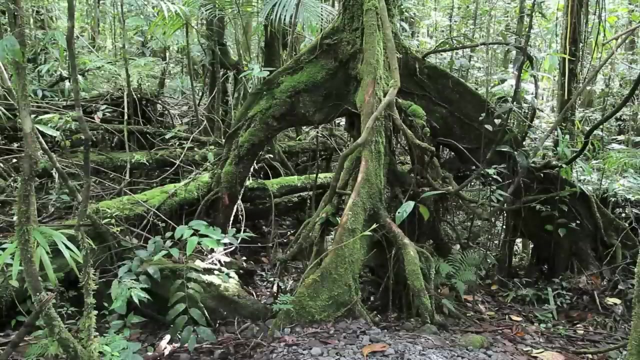 the study of life. The biosphere is made up of many different biomes. Biomes are regions of plants, animals and other living things that have adapted to live in that particular region's terrain and climate. Deserts and forests are types of biomes. So are rainforests, grasslands and wetlands. 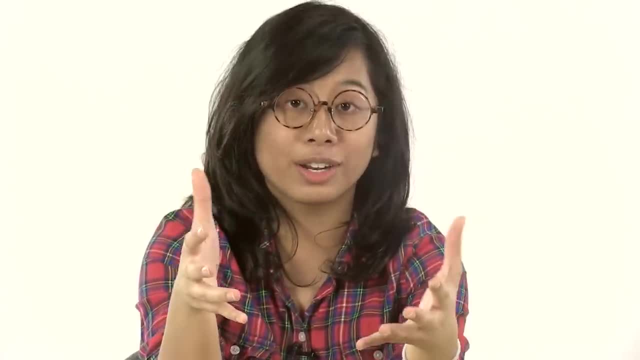 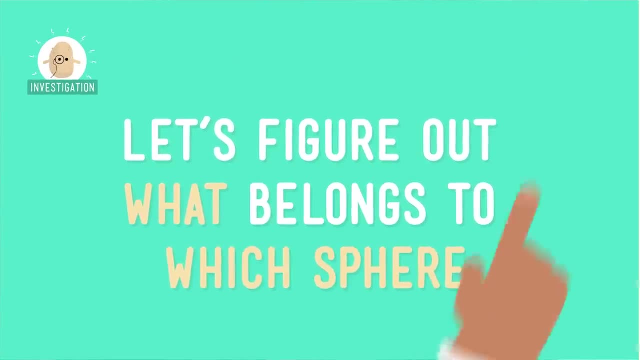 All of these biomes, and many more make up the biosphere. Okay, now that we know what's in these two spheres, let's put them together and try to figure out what belongs to which sphere. Imagine a lovely forest meadow. 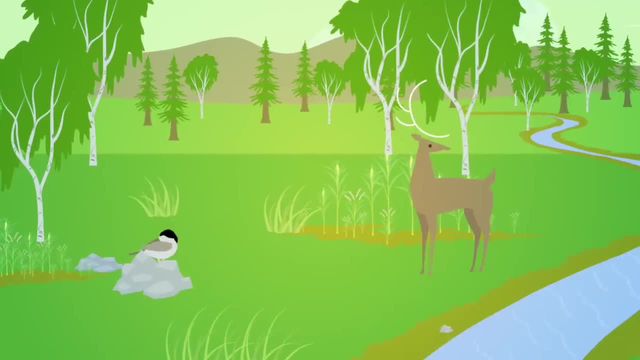 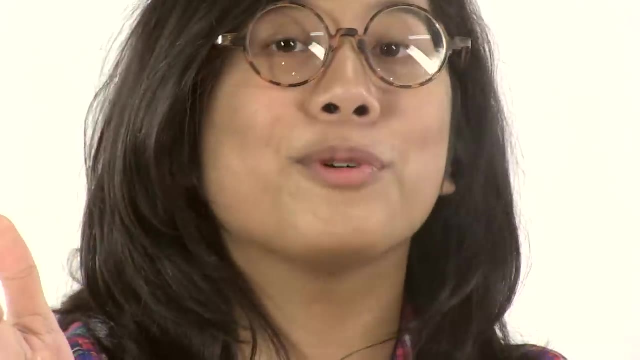 A bird perched on a rock chirping away, A deer standing in the tall grass, A mountain standing tall in the background in a stream flowing through the clearing. Ah, I can almost smell it. Almost everything in this scene is part of either the geosphere or the biosphere. Let's 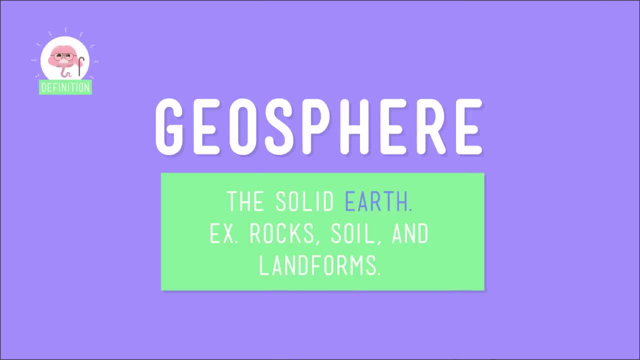 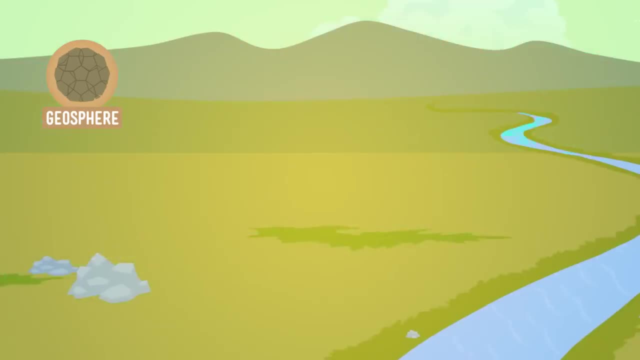 see if we can figure out which parts go into which sphere. Let's start with the geosphere. We know that there's nothing alive in the geosphere, so we can rule out all the plants and animals. Water is also part of a different sphere. 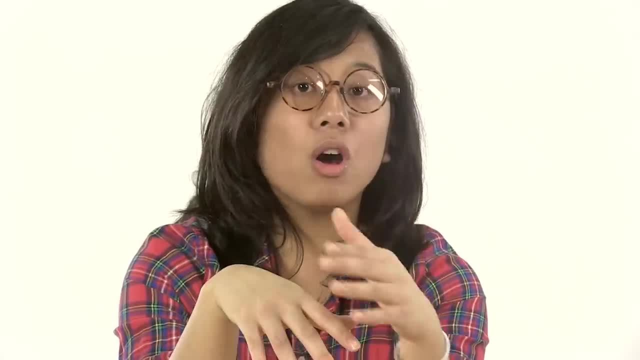 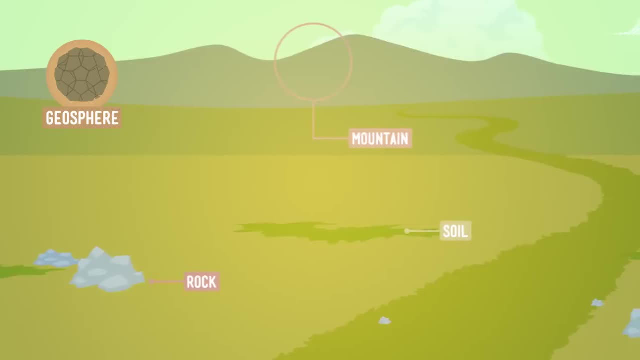 but we'll talk about that later. When we take away the living things, we're left with all the solid earth parts of the scene: The rock, the bird was standing on the soil, the grass was growing out of the mountain in the distance and the bed, the stream. water flowed through.